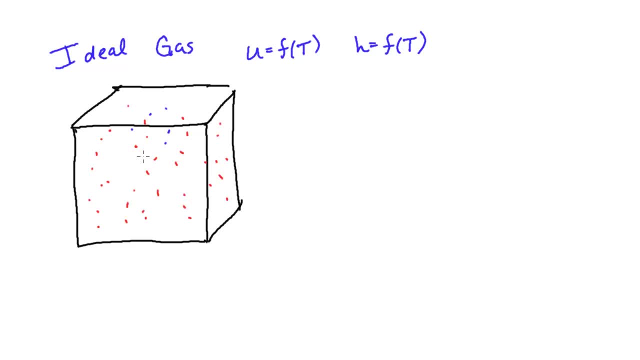 And we have blue water vapor molecules. Now, actually, there's a lot more empty space than this in reality. when you talk about gases in a room, This visual will have to do Do justice. If we have this, the total pressure in that room exhorted by all the molecules is just the sum of the dry air molecules and the water vapor molecules. 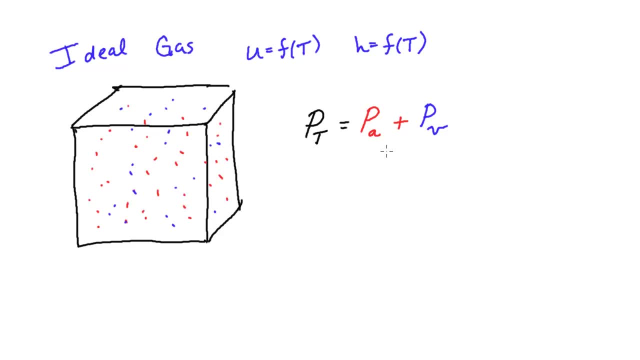 So they exist as if they knew nothing of the other, Completely independent. And so we know also that We have Both of them are ideal gases and obey the ideal gas law. So we have the partial We call. it calls the partial pressure of air and the partial pressure of vapor and the total pressure of the air. 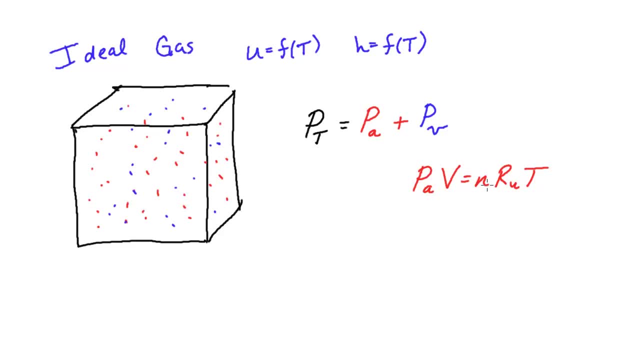 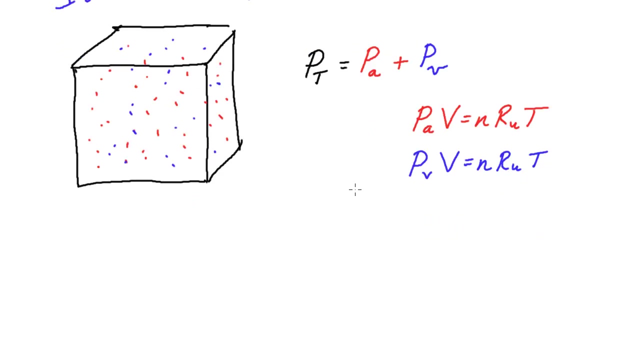 Well, the partial pressure of air times, the volume of the space times, the number of molecules and universal gas constant, The absolute temperature. that holds for dry air and That same relation Also holds For the water vapor that's in the air. And what I want to cover in this video is to say: OK, we have water vapor in the air. 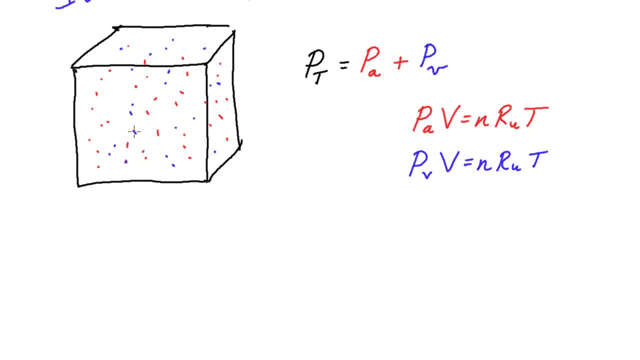 What's a good Measurement or property or value that we can discuss with other people in HVAC about? Well, is it got a little water in the air? Is it have a lot of water in the air? What's a good Measure of that? 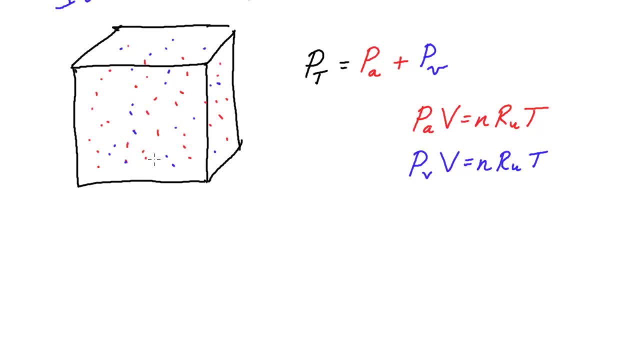 Well, we have mass. Mass is a good measure of the amount of stuff, So a semi intuitive Way of describing how much water vapors in the air is to. Let's compare the mass of the water vapor compared to the mass of the dry air. 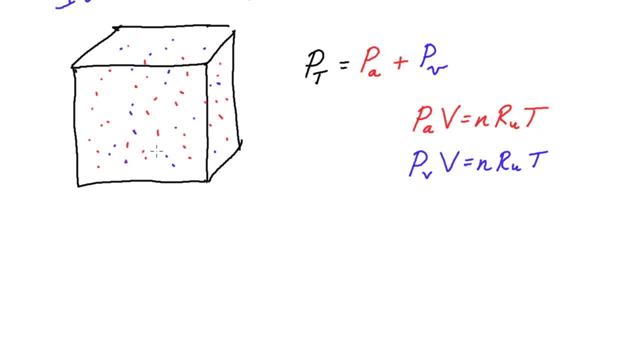 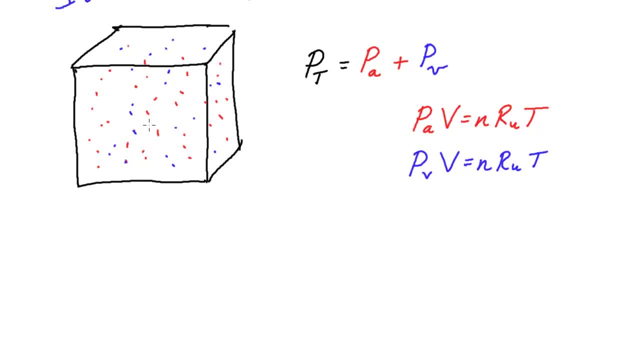 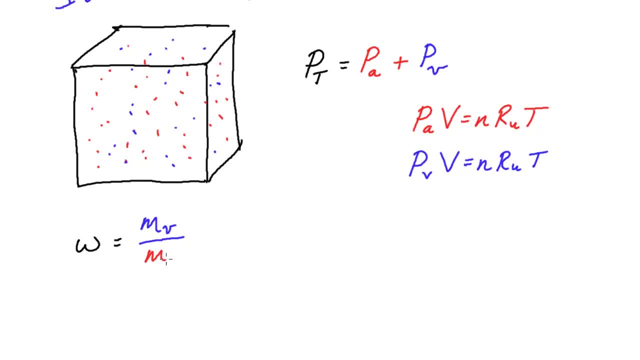 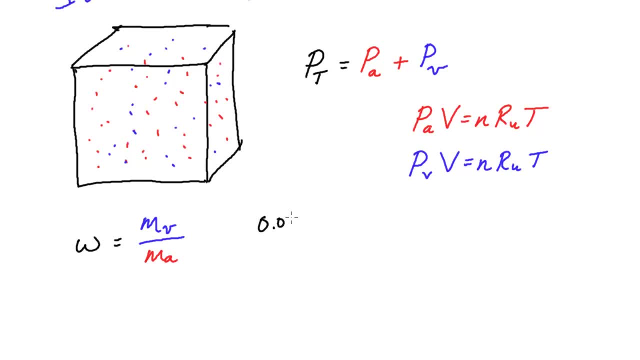 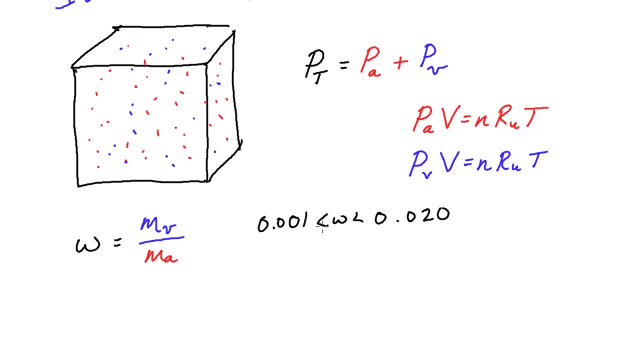 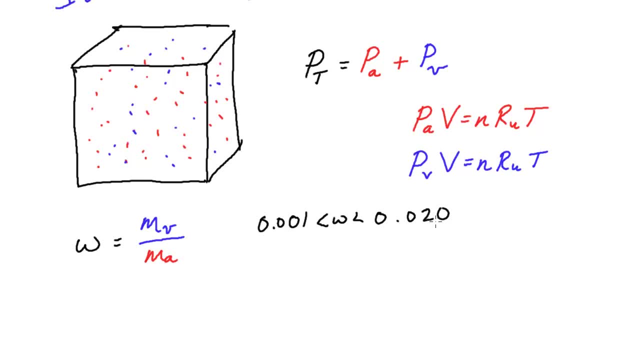 Let me, Let me, Let me water vapor and in fact, for the majority of the time, it's less than that. Now we have this relationship and this is nice, but it's also nice to have this measure of absolute humidity, or they call it specific humidity, in terms of things we can measure. 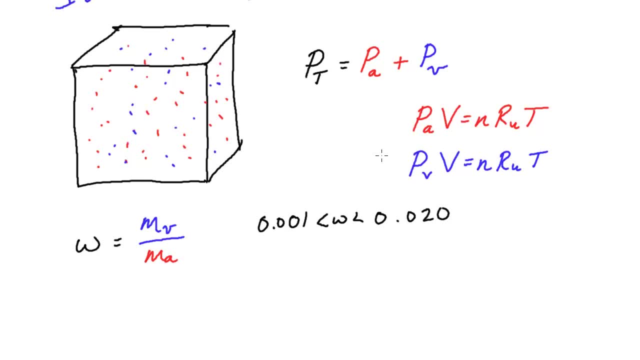 and what can we measure? We can measure pressure. Mass of the water vapor is a little hard to measure, but we can measure pressures and we understand partial pressures and the saturation pressures that we have tabulated in the thermodynamics books. So lets use these relations to take this formula for omega and lets put it in terms of pressure. 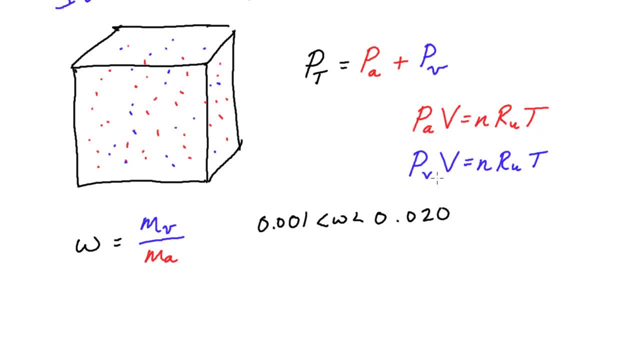 So one of the first things we have to do is we need to go ahead and take one of these equations and we need mass in this equation. Fortunately, what we have is we know that If we take, we have something called the specific gas constant, that's, the universal gas constant. 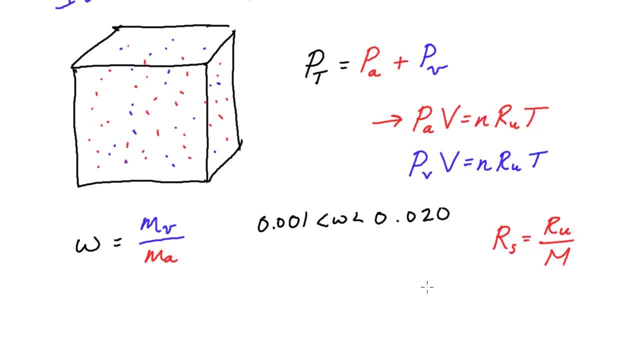 divided by its molecular mass. We also know that the mass is the molecular mass multiplied by the number of molecules. So if we take this equation and we do some substitution, So instead of n I'm going to put the mass over the molar mass- times the universal gas. 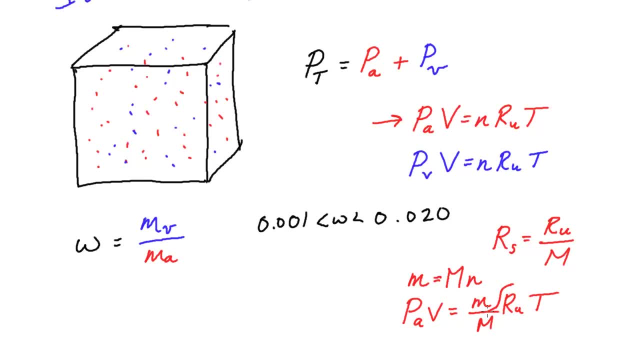 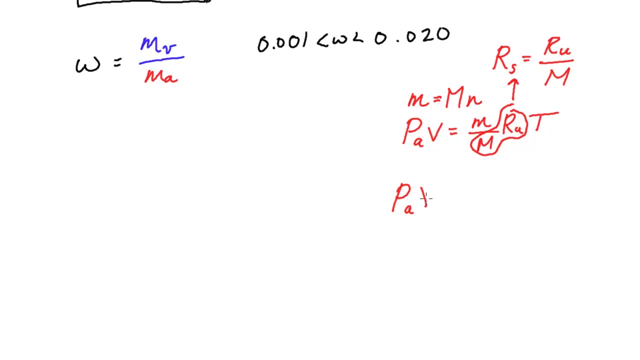 constant times: temperature. If you realize that this here is the specific gas constant, then we can rewrite this a little bit. So let me scroll down and let's rewrite this So we have partial pressure. dry air times. the volume of the space mass of the dry air. 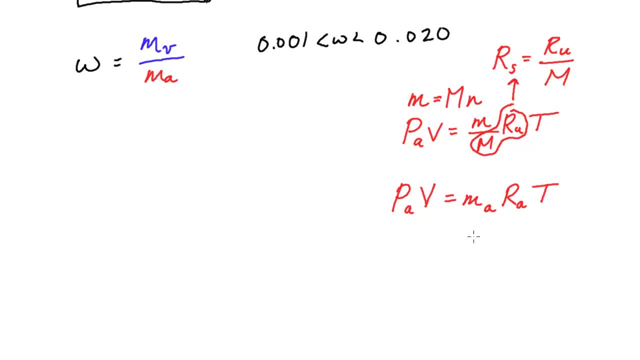 specific gas constant of dry air times, temperature, and then we can solve for the mass of the air. So that's simply partial pressure of air volume, specific gas constant and temperature, And we can do the same thing for water vapor, just these subscripts will change. 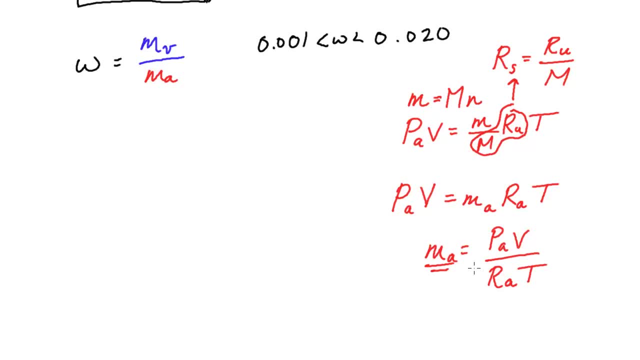 So we have this relationship. we'll have one exactly for the same for water vapor. So let's go back to our original formula and let's substitute these things. So we have: omega is equal to draw a fraction bar on the vapor side we have on the top. 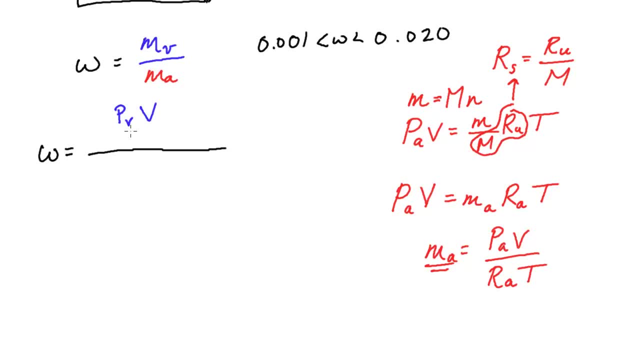 of the fraction. we have P vapor volume divided by R vapor temperature. on the bottom we have that relationship to the bottom right And so now we can start simplifying and if you notice right away, some things are going to cancel. Cancel with that. that T is going to cancel with that. 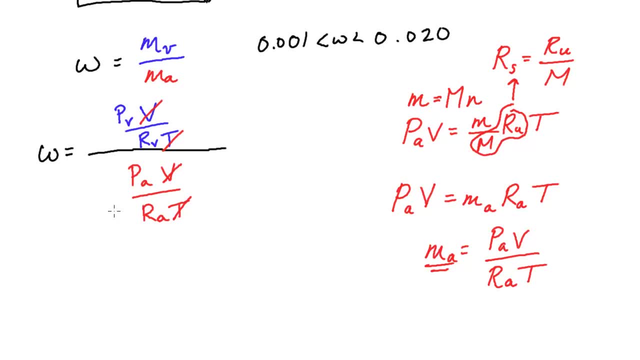 And if you can kind of do this mental fractional arithmetic, Let's move down here. we have omega is- let me do that in color- is P V over R V, and we have R A and P A. So that's nice. but what's also interesting is we know this value here and we know this: 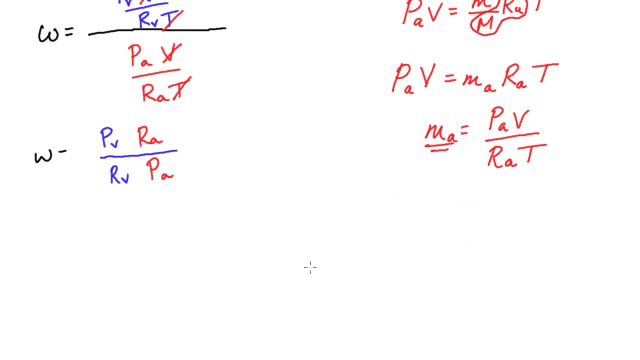 value. here we can go look up these values. So let's just remind ourselves of what the specific gas constants are. so if we have the gas constant for air, It's equal to divided by the molecular mass of air, and this gas constant is 8.314 kilojoules per kilomole Kelvin. 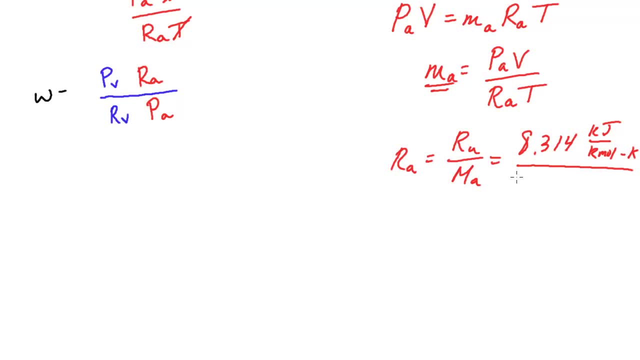 And if you would go look up online or in some resource, the molecular mass of air is somewhere on the order of 28.96 kilograms per kilomole And if you were to do this calculation you'd get something on the order of 0.287.. 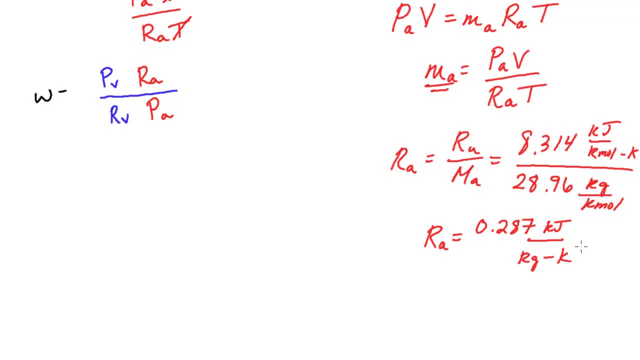 Kilojoules per kilogram Kelvin. these cancel. this goes on the bottom of the fraction. And if we do this for water vapor, again 8.314 kilojoules per kilomole Kelvin. And water vapor is for the most part oxygen: one oxygen, two hydrogens, 16.. 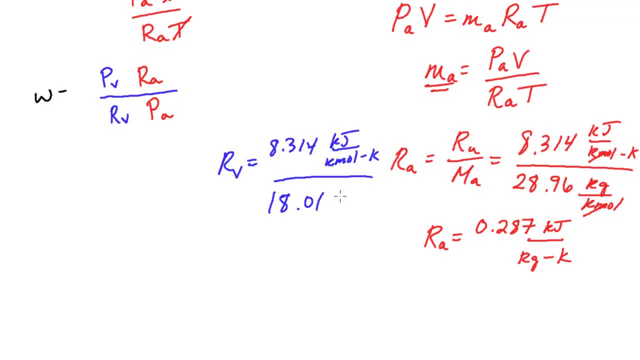 And they might throw an extra 0.01 to this just for good measure. but you have oxygen, which is 16,, and hydrogen, which is one each two of those kilograms per kilomole. If you do that, you would get something on the order of- let me get my calculator: 0.462 kilojoules per kilogram Kelvin. 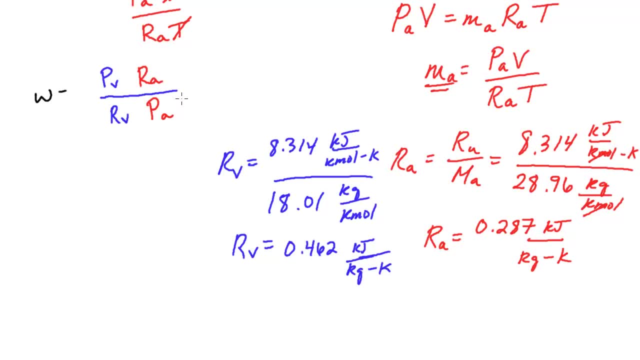 So now we have these two values and we can actually do this division, And so if you actually take that 0.287 and divide it by 0.462, you will get something that is close to 0.622.. And we still have the partial pressure of the vapor on the top of this fraction. 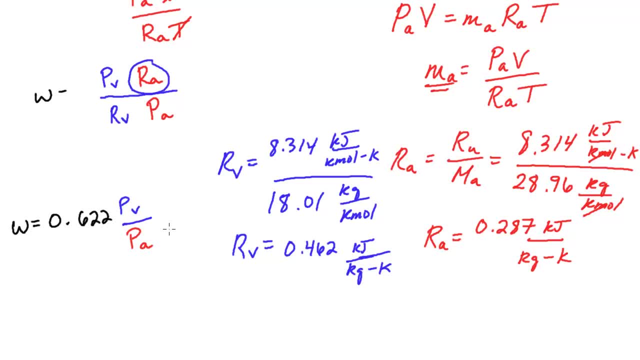 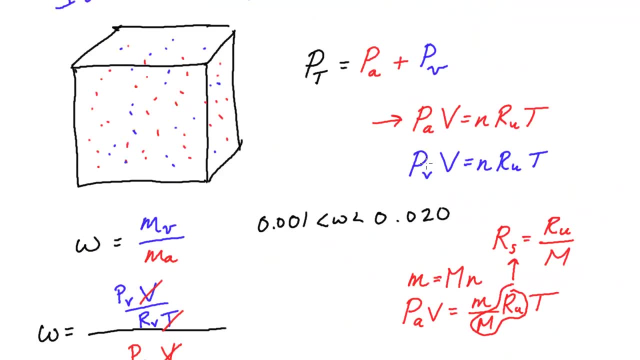 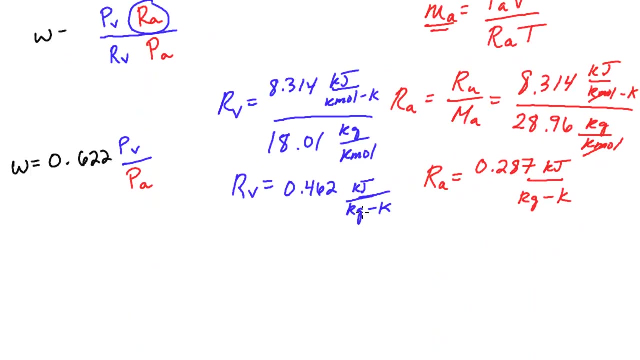 Divided by Partial pressure of the dry air. And in some textbooks now you'll see we already knew from earlier that the total pressure was dry air plus the vapor pressure. If we come down here we know: if we move this to the other side of the equation, we have total pressure minus vapor.